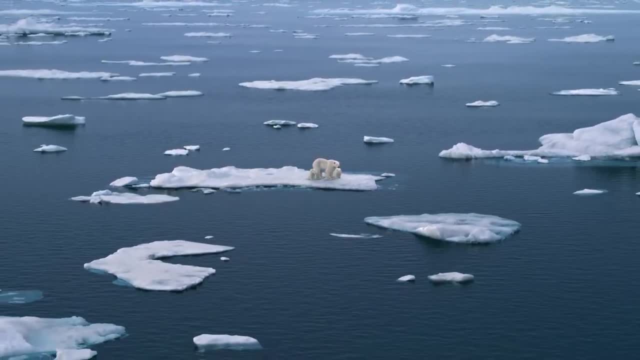 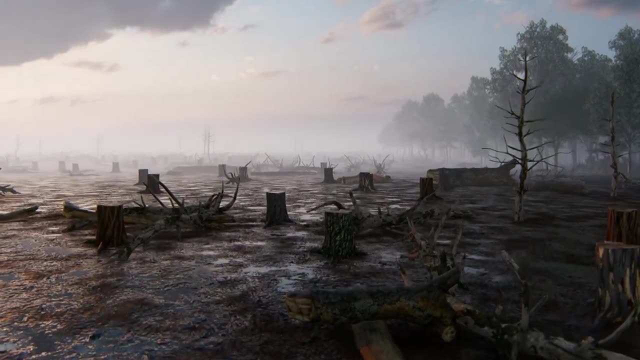 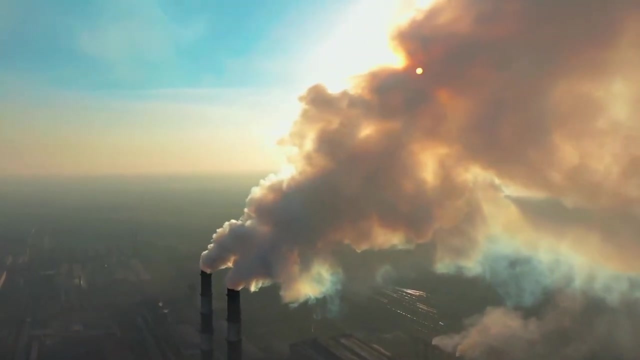 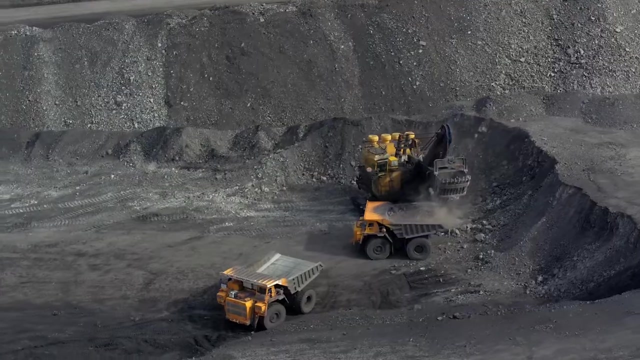 and organisms that inhabit them. Sadly, scientists have also confirmed that this warming of the earth is due to increased greenhouse gases in the atmosphere caused by human activities. A main cause of increased greenhouse gases in the atmosphere is the burning of fossil fuels like coal. 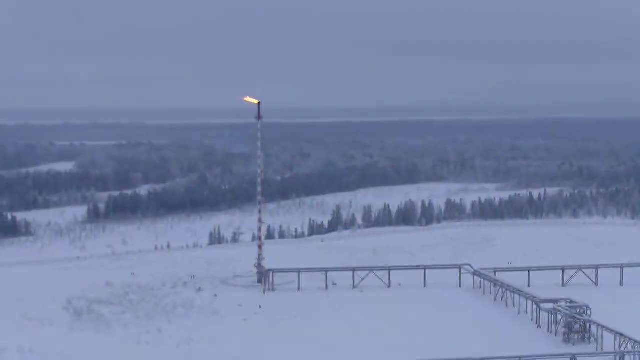 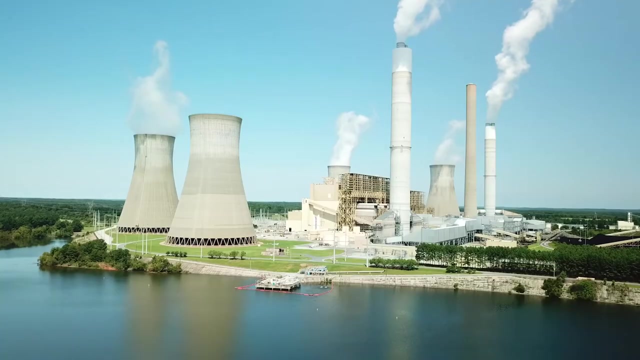 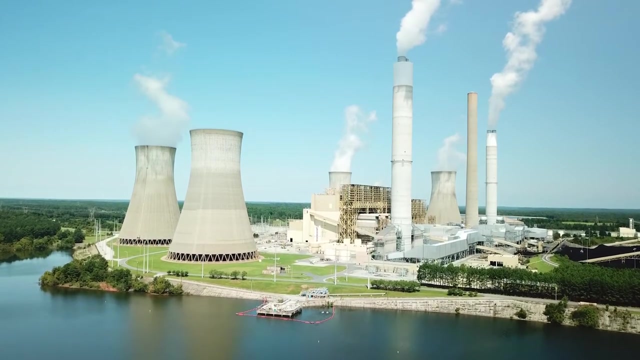 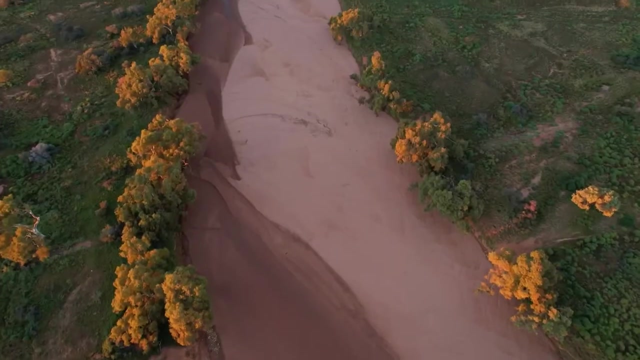 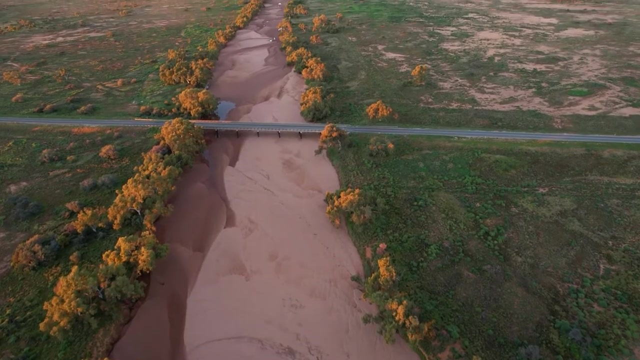 oil and gas. Burning fossil fuels in vehicles, manufacturing and to produce electricity releases carbon dioxide and other pollutants into the air. This causes the atmosphere to trap more heat, resulting in a warmer earth. This process is now referred to as human induced climate change. 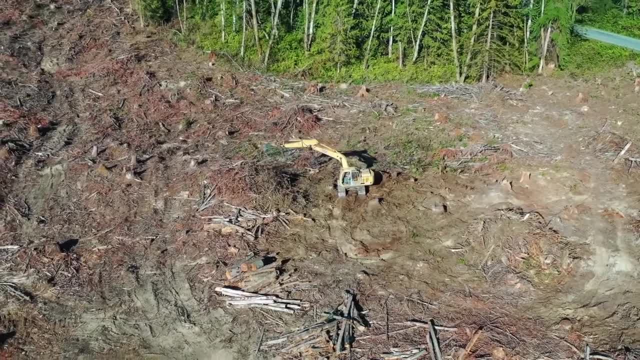 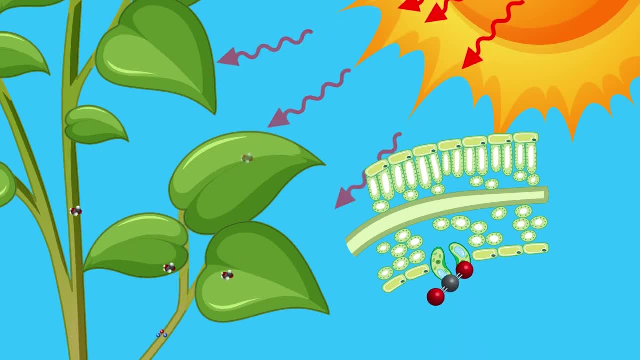 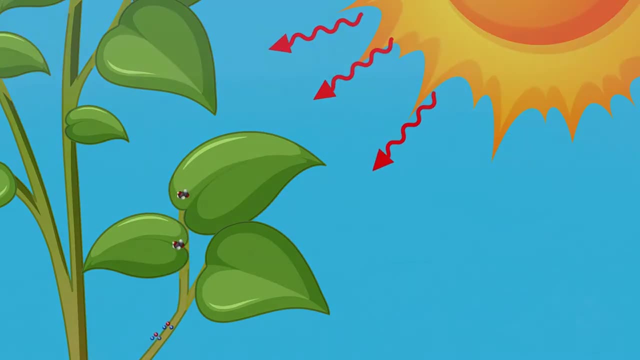 Also contributing to human induced climate change is deforestation. When plants photosynthesise, they take in carbon dioxide from the air, making them a major source of carbon dioxide removal from the atmosphere. When we clear forests to make ways for cities and farming, the vegetation that was once 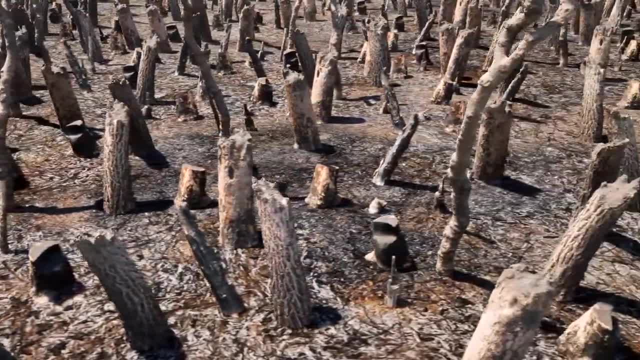 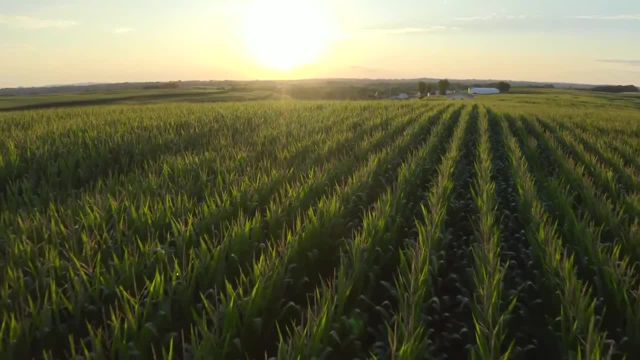 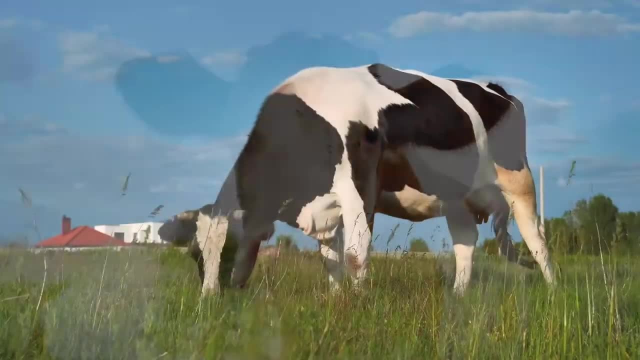 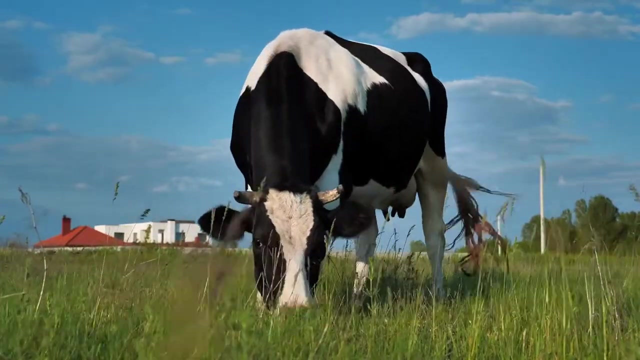 there can no longer remove carbon dioxide from the air. There is another surprising contributor to human induced climate change. These guys- Cows- are used by people all over the world As a source of meat and dairy products. When cows digest their food, they produce methane gas, which you may recall, is also 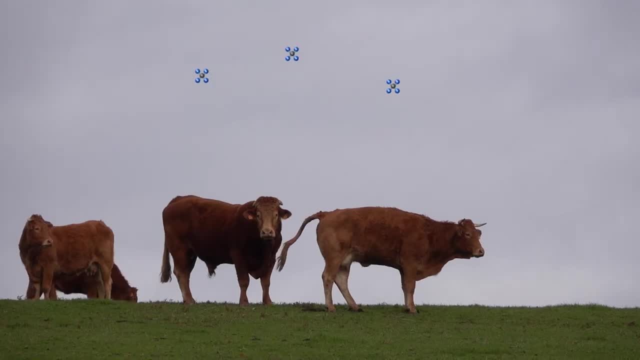 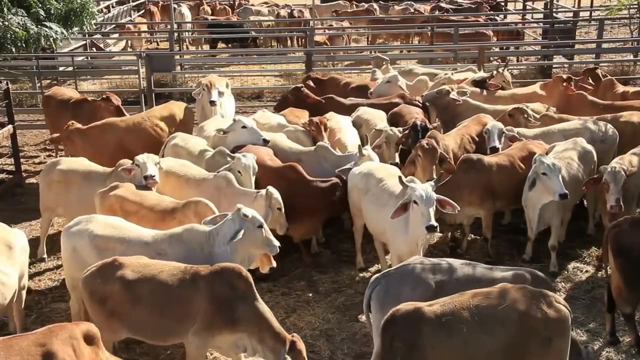 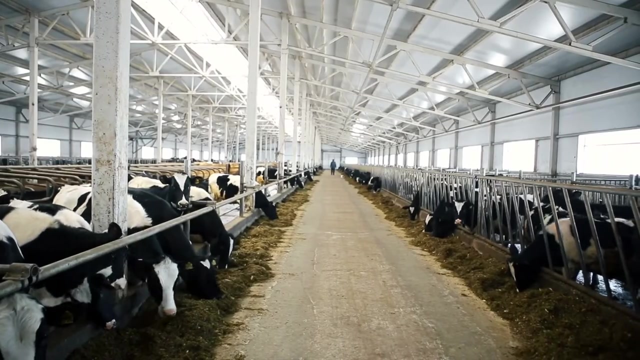 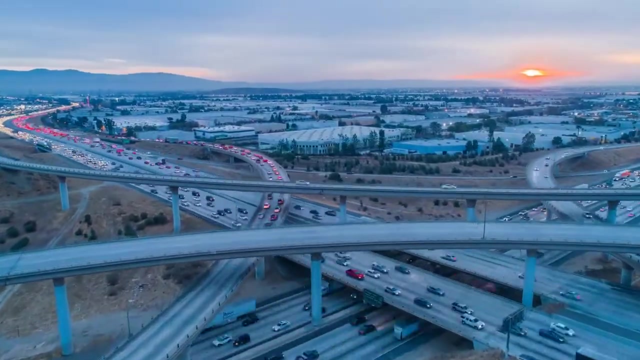 a greenhouse gas. The gas from a few cows would normally not be reason for concern. The problem comes when humans farm over a billion cows a year, and with the human population increasing, so too is our demand. The impacts of human induced climate change are far reaching and complex. 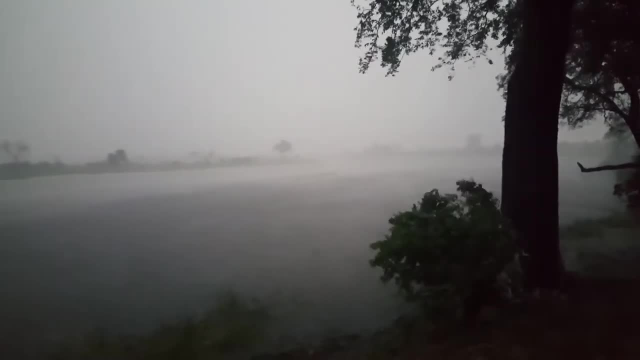 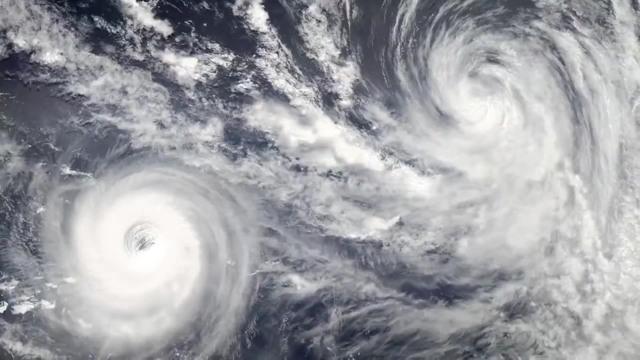 They include, but are not limited to, alterations in precipitation, sea level changes, ocean acidification and more extreme weather events. These changes pose serious risks to all of us. We are all in this together. We are all in this together. We are all in this together.